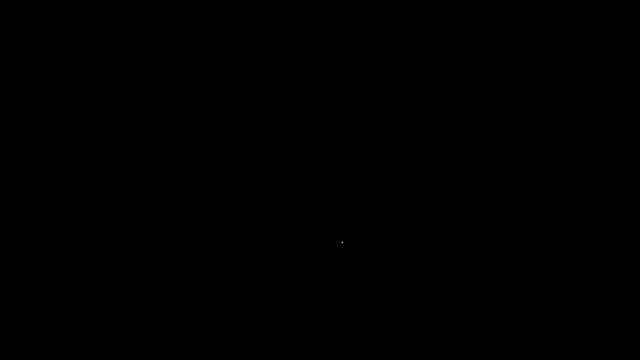 In this video we're going to focus on permutations and combinations. But what exactly is a permutation and how is it different from a combination? A permutation is associated with arranging things in different order: Combinations: you simply concerned about combining things. For a permutation, the order. 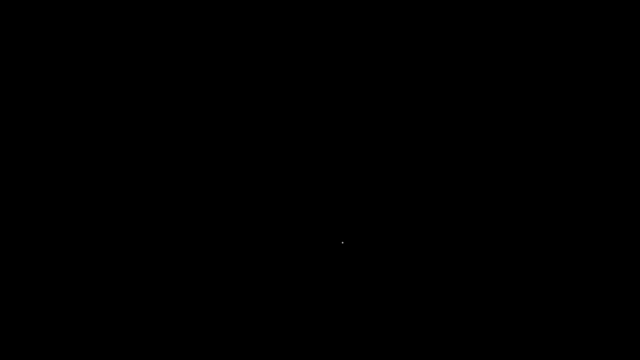 matters, but for a combination the order does not matter. I guess the best way to explain this is with an example. Let's say, if we have three letters ABC, We could arrange them in this order: ABC. or we could say CAB. Now, even though we have 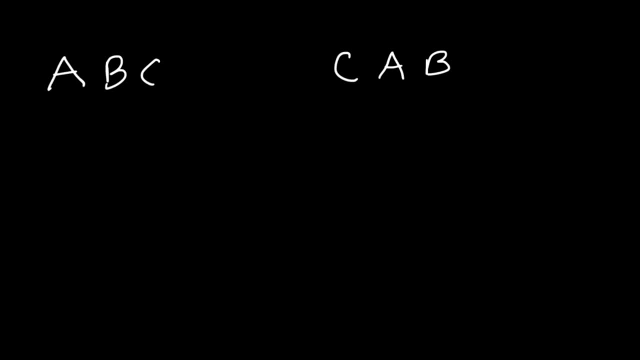 the same three letters. the order is different. So these are two different permutations. The number of permutations is two, However, the number of combinations is one. These two are considered to be the same in terms of a combination, But in terms of a permutation they're considered to be two separate things. So just make sure you. 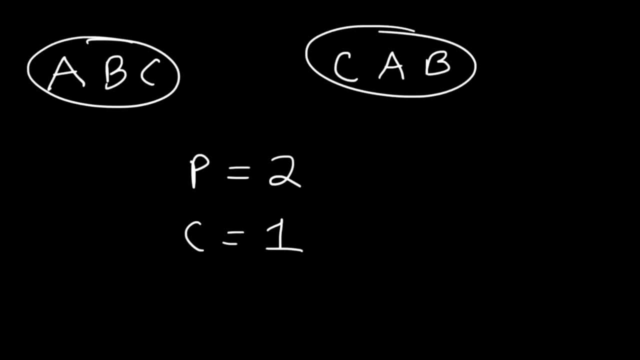 understand that a permutation, the order matters, The way you arrange it matters. And for a combination the order doesn't matter, You just want to combine things. So if you have ABC and CAB, you still have the same three letters combined in a group. So for a combination they're the same. 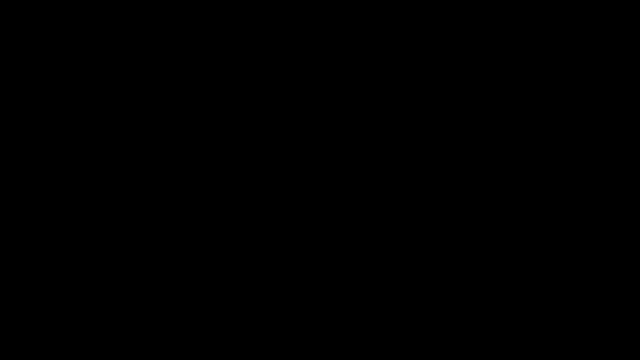 Let's use another example to illustrate this. Let's say, if we have four letters- A, B, C and D- And let's choose two of the four letters, In how many different ways can we arrange two of the four letters? And also, how many different ways? 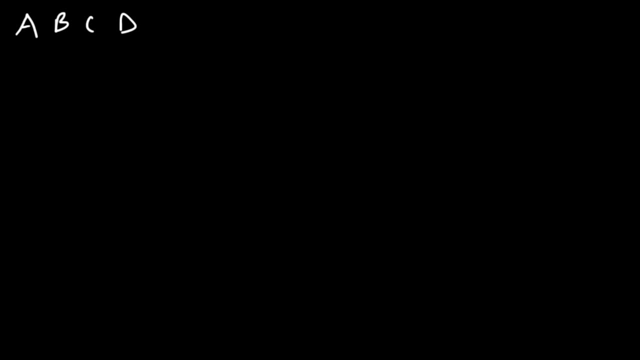 can we combine two of the four letters And use that to determine the number of permutations and combinations of choosing two out of the four, And then we'll talk about how to use an equation to get that same answer. So we can choose AB, we can choose AC or we could. 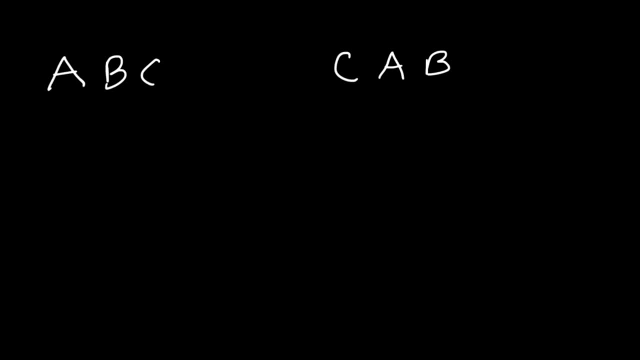 the same three letters. the order is different. So these are two different permutations. The number of permutations is two, However, the number of combinations is one. These two are considered to be the same in terms of a combination, But in terms of a permutation they're considered to be two separate things. So just make sure you. 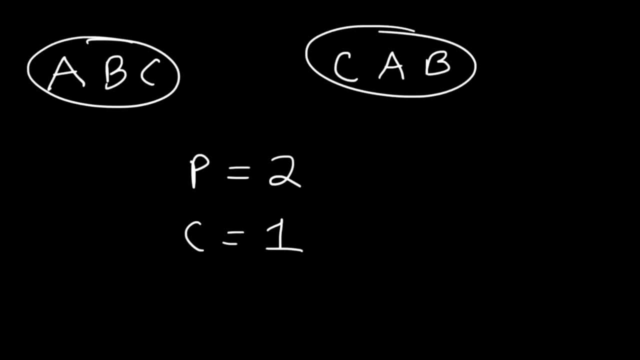 understand that a permutation, the order matters, The way you arrange it matters. And for a combination the order doesn't matter, You just want to combine things. So if you have ABC and CAB, you still have the same three letters combined in a group. So for a combination they're the same. 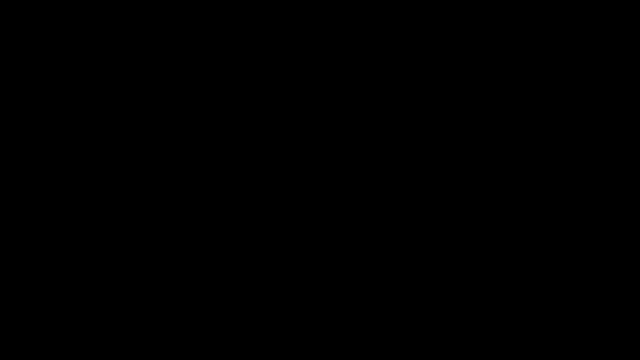 Let's use another example to illustrate this. Let's say, if we have four letters- ABC and D- And let's choose two of the four letters, In how many different ways can we arrange two of the four letters? And also, how many different ways can we? 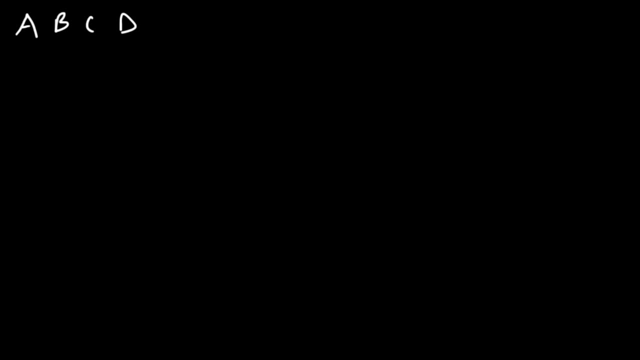 combine two of the four letters And use that to determine the number of permutations and combinations of choosing two out of the four, And then we'll talk about how to use an equation to get that same answer. So we can choose AB, We can choose AC, Or we could. 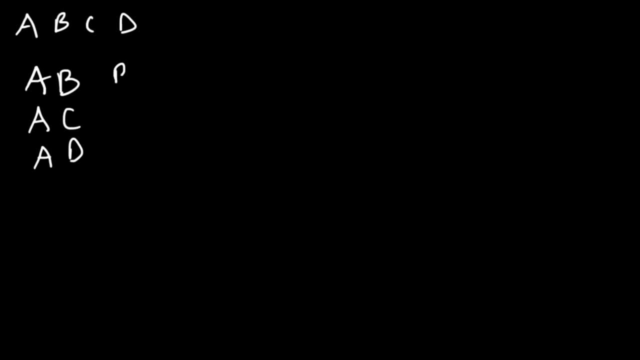 choose AD. We can choose BA, BC, BD. We're only using each letter once. every time we select two out of the four. We can also use CA, CB and CD, And also DA, DB, DC. So notice that there's a total of 12 different ways. we can arrange two out of the four letters. 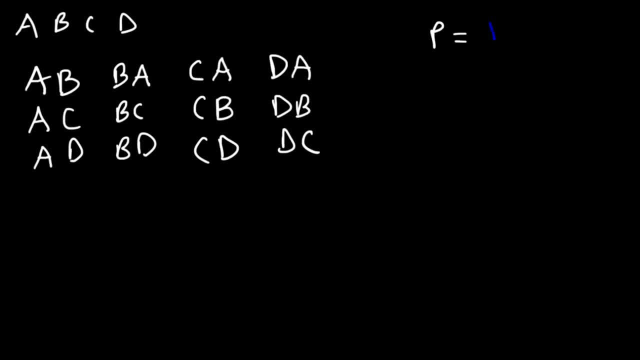 So the number of permutations in this example is equal to 12.. Now, what about the combinations? So the number of permutations in this example is equal to 12.. Now, what about the combinations? Now, if you recall, for a combination, the order. 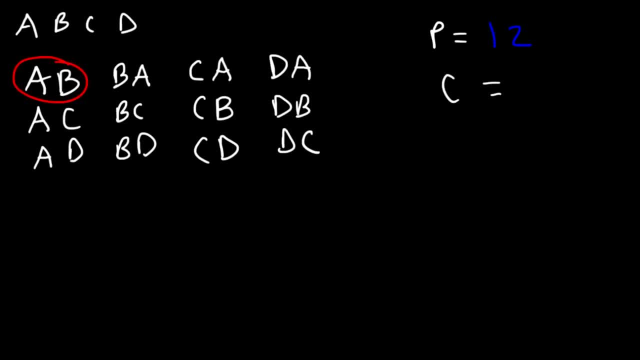 doesn't matter. So take a look at AB and BA. In terms of permutations, these are counted as two separate things, But for a combination, you're combining the same letters and since the order doesn't matter for a combination, they're counted. 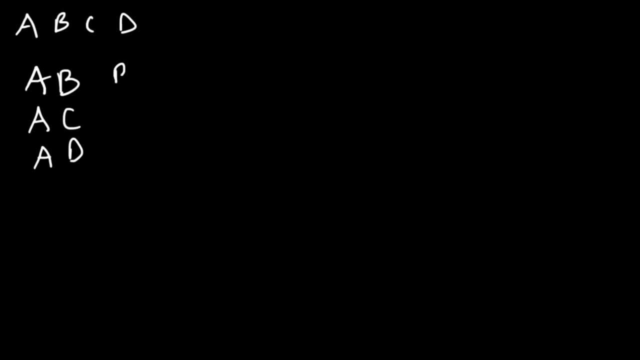 choose AD. We can choose BA, BC, BD. We're only using each letter once every time. we select two out of the four. We can also use CA, CB and CD, And also DA, DB, DC. So notice that there's a total of 12 different ways. we can arrange two out of the four. 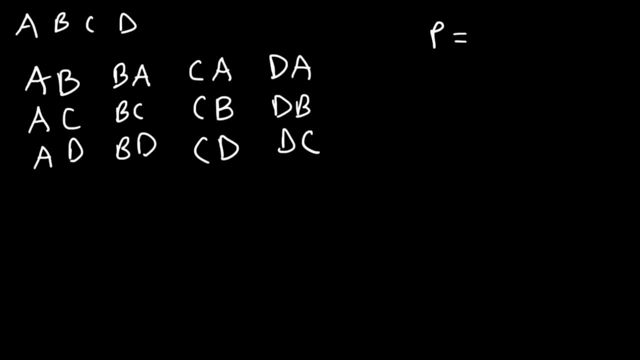 letters. So the number of permutations in this example is equal to 12.. Now, what about the combinations? Now, if you recall, for a combination the order doesn't matter. So take a look at AB and BA. In terms of permutations, these are counted as two separate things. But 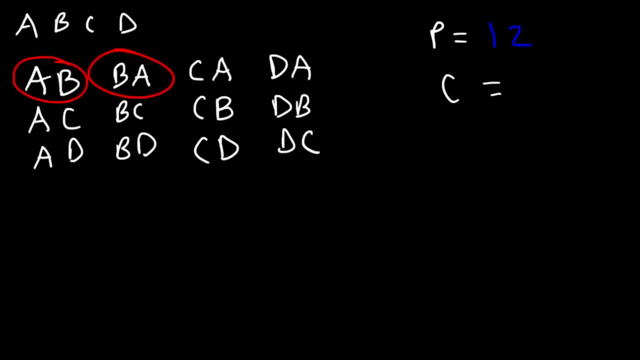 for a combination, you're combining the same letters And since the order doesn't matter for a combination, they're counted once as a combination. So if we're going to count AB, we can't count BA. If we're going to count, 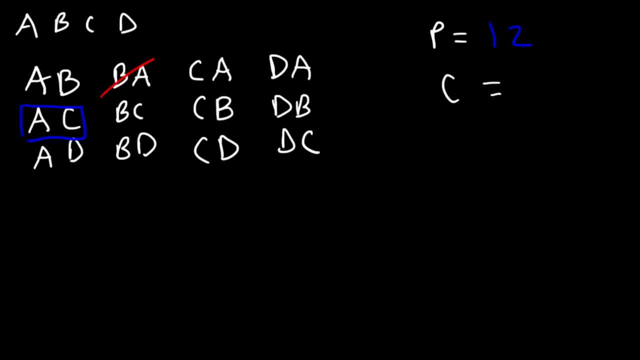 let's say AC, we can't take into account CA. if we're going to count AD, we have to eliminate DA. if we're going to use BC, we need to get rid of CB. if we're going to use BD, we can't use DB. and finally, if we're going to use CD, we got to get rid. 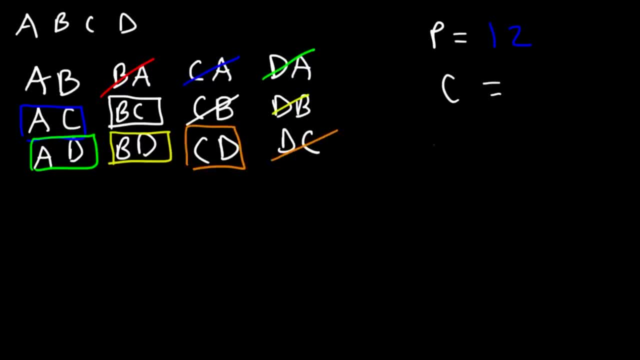 of DC. so notice that the number of combinations is equal to six: one, two, three, four, five, six. so now you can clearly see the difference between a permutation and a combination. so just remember: a permutation, the order matters, and for combination, the order does not matter. now how can we calculate these? 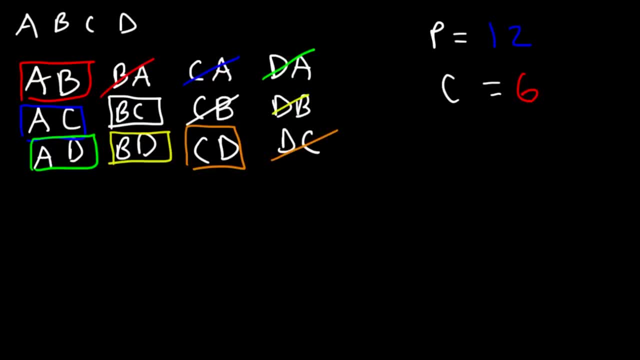 answers. is there an easier way to in which we can find a value, as opposed to making a list of all the different possibilities? the first equation you need to know is NPR. this helps you calculate the permutations. now there's four letters and we're choosing two, so 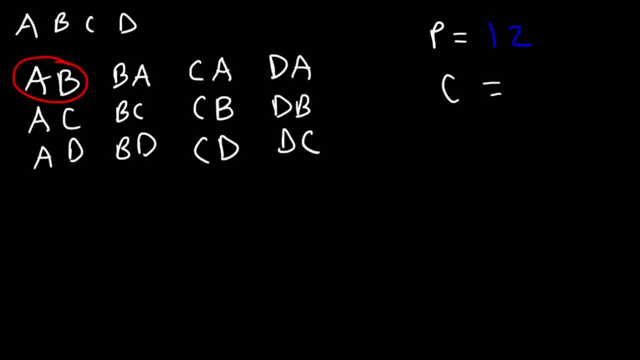 once as a combination. So if we're going to count AB, we can't count B, A. If we're going to count, let's say, AC, we can't take into account CA. if we're going to count AD, we have to eliminate DA. if we're going to use BC, we need to get rid. 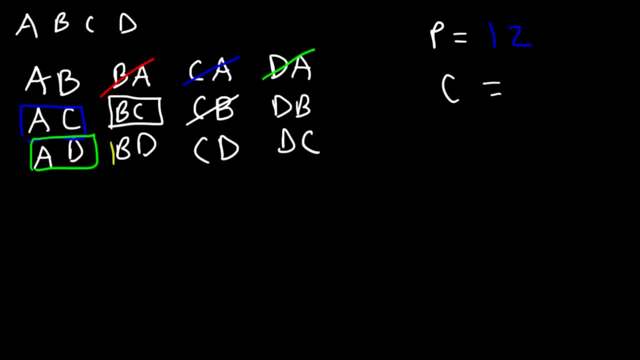 of CB. if we're going to use BD, we can't use DB. and finally, if we're going to use CD, we got to get rid of DC. so notice that the number of combinations is equal to 6: 1, 2, 3, 4, 5, 6. so now you can clearly see the difference between a. 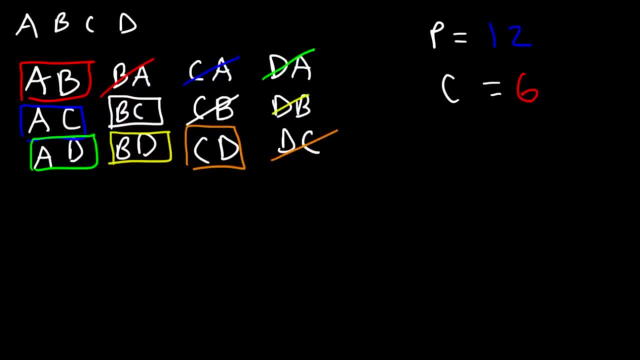 permutation and a combination. so just remember: a permutation, the order matters, and for combination, the order does not matter. now, how can we calculate these answers? is there an easier way in which we can find a value, as opposed to making a list of all the combinations that we need to take into account to get rid of? 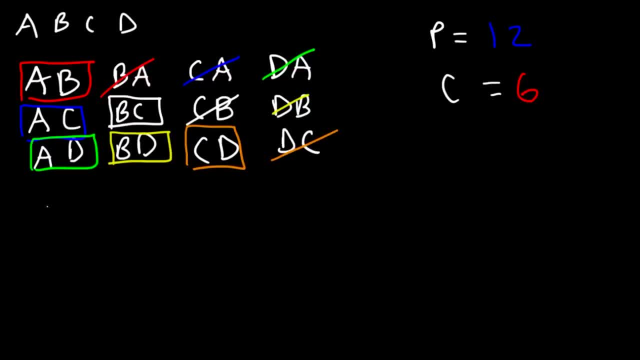 the list of all the different possibilities. the first equation you need to know is NPR. this helps you calculate the permutations. now there's four letters and we're choosing two, so it's going to be 4 P 2. we're choosing two out of a group of four. now the equation NPR is equal to N factorial divided by. 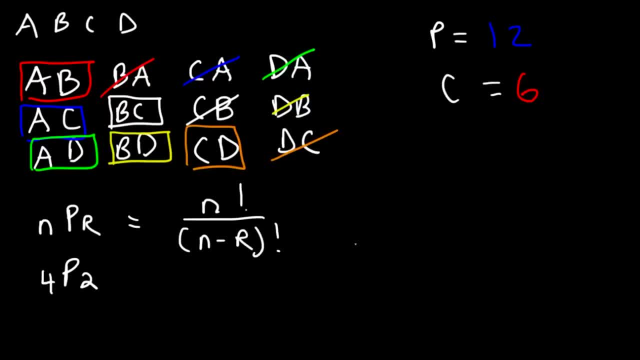 N minus R- factorial. in this case, we can see that the number of combinations is equal to 4 P 2. we're choosing two, so it's going to be 4 P 2. we're choosing two, so N minus R, that's going to be 4 minus 2. now, 4 minus 2 is 2, so we have 4. 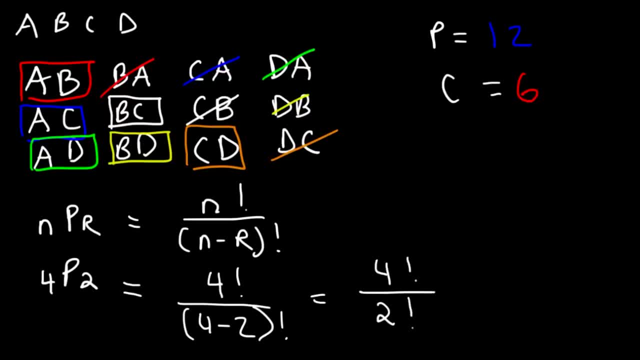 factorial divided by 2 factorial. so what exactly is 4 factorial? 4 factorial is 4 times 3 times 2 times 1. you start with this number and you multiply 4 by every integer all the way to 1. 2 factorial is simply 2 times 1, so we can cancel 2 times. 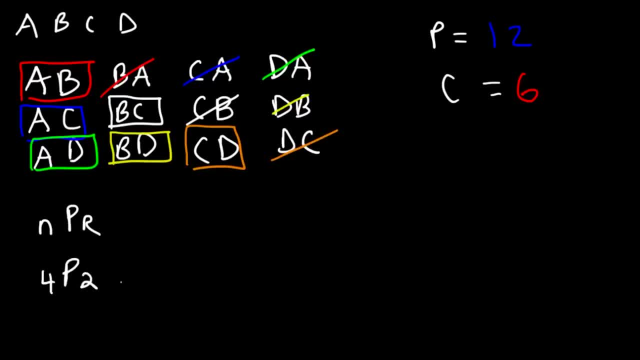 it's going to be four P two. we're choosing two out of a group of four. now the equation: NPR is equal to n factorial divided by. NPR is equal to n factorial divided by n minus R factorial. in this case we can see that n is four and R is two, so n. 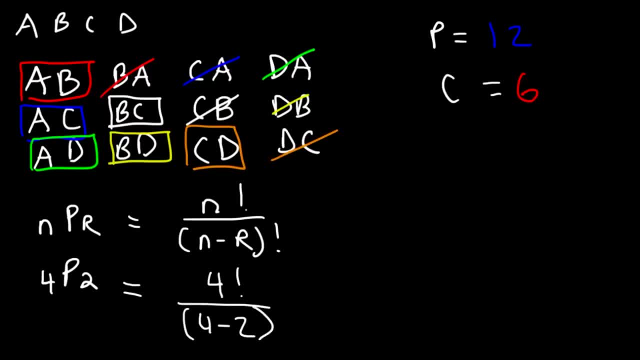 minus R, that's going to be four minus two. now, four minus two is two. so we have four factorial divided by two factorial. so what exactly is four factorial? four factorial is four times three times two times one. you start with this number and you multiply four by every integer, all the 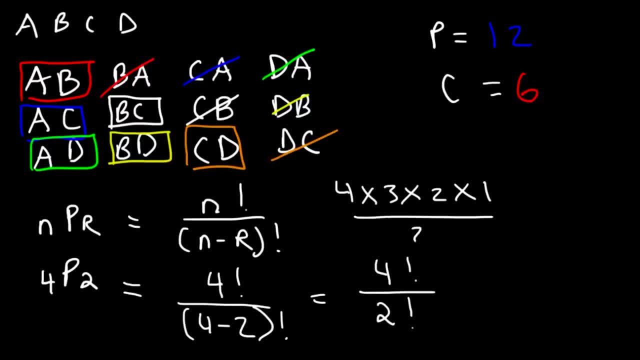 way to 12. factorial is simply two times one, so we can cancel two times one and we're left with four times three, and we know that four times three is equal to 12, which is what we have here. now how can we calculate the combination? what is the formula that we can use? 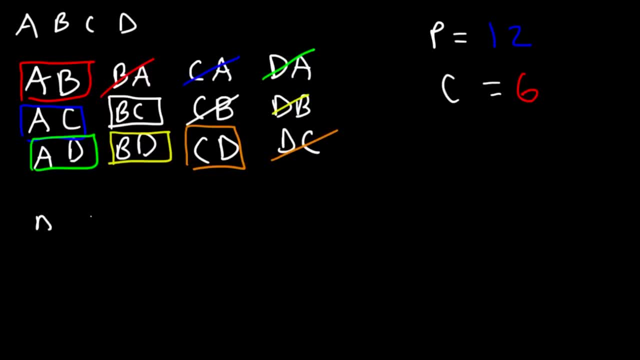 NCR is equal to n factorial divided by n minus R factorial divided by R factorial. so basically, in terms of a permutation, a combination is equal to NPR divided by R factorial- this portion right here is NPR- and then divided by R, NCR is equal to NPR divided by R factorial- this portion right here is NPR- and then divided by R. 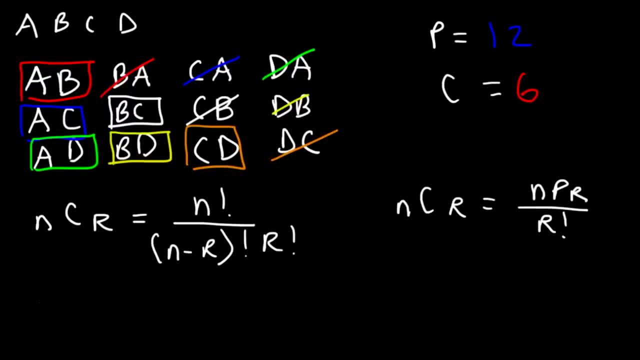 so we have four c2 in this example. so n is four and R is two. so this is equivalent to four factorial divided by two factorial times two factorial. and we know that four factorial is four times three times two times one. two factorial is two times one and we have another two factorial. it turns out that two times. 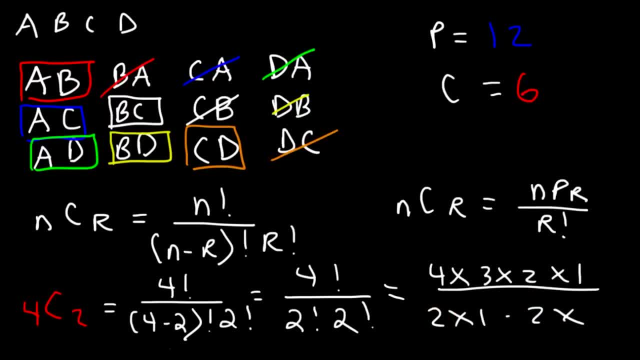 two is four, so we could cancel those twos. with the four on top we could ignore one, because one times anything won't change the value. so what we have left over is three times two. three times two is equal to six, and so now you understand how to. 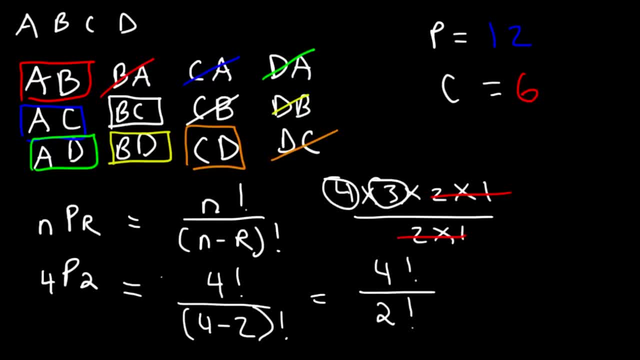 1 and we're left with 4 times 3, and we know that 4 times 3 is equal to 12, which is what we have here now. how can we calculate the combination? what is the formula that we can use? and see our raise, our Shane Lipschitz, and we call it crazy. 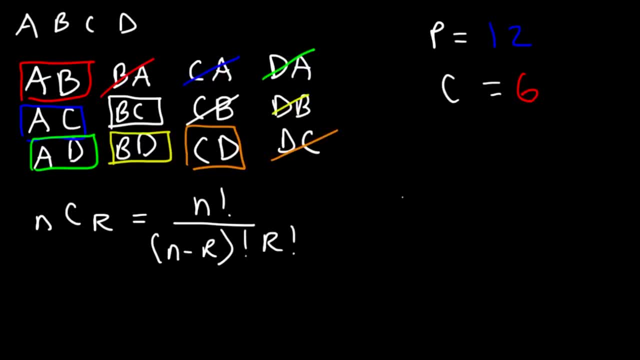 this is a formula that we use to calculate nonlinear functions. so we have four and six-strang commun Republicans and we couldn't calculate six-strang commun 먹을 and two-strang commun Republicans, and we really needed to remember one thing is: we can't always obtain gauging, ноS guardians can are. like adults, one can get an favors from a nation and one can't get value from a nation. so I'd like to comment on a method we use to calculate sonar and not a index of this. P Dublin n is equal to N factorial divided by N Minus r factorial divided by r factorial. so basically, in terms of a permutation accommodation is equal to NPR divided by r factorial. this portion right here is NPR and then divided by R. so we have four and six-strang commun Republicans and we have four inditanians. we will evaluate to to a problem which we have created in the last chapter. 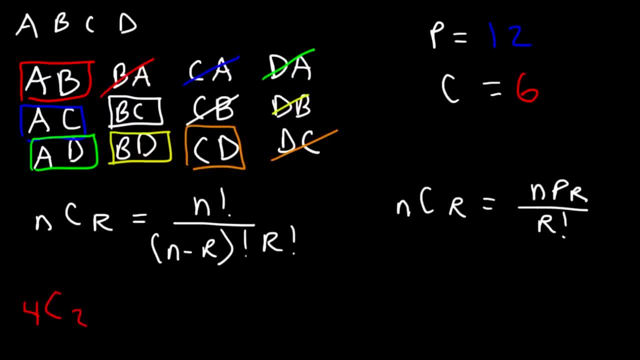 C2 in this example. So n is 4 and r is 2.. So this is equivalent to 4 factorial divided by 2 factorial times 2 factorial, And we know that 4 factorial is 4 times 3 times 2 times 1.. 2 factorial is 2 times 1 and we have another 2 factorial. 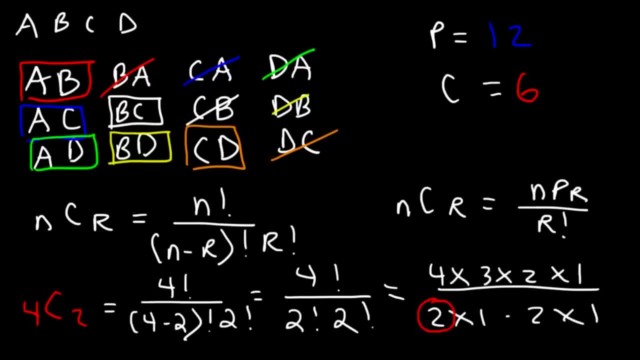 It turns out that 2 times 2 is 4.. So we could cancel those 2's. with the 4 on top, We could ignore 1, because 1 times anything won't change the value. So what we have left over is 3 times 2.. 3 times 2 is equal to 6.. And so now you understand how to use. 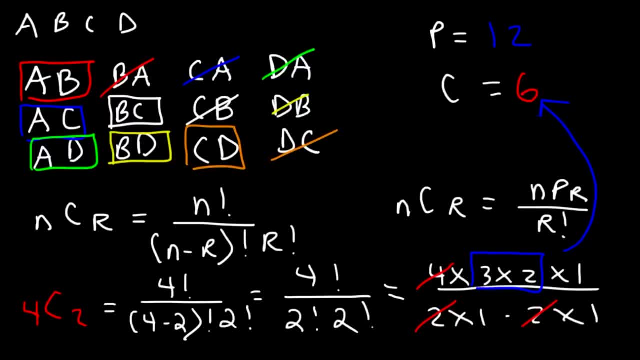 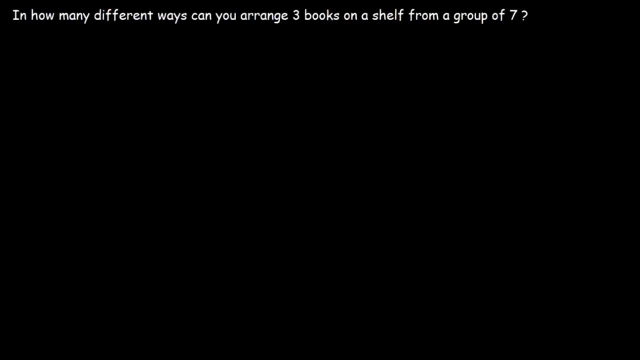 the equation and also you understand how to make a list to determine the number of permutations combinations. So now let's work on some example problems. In how many different ways can you arrange three books on a shelf from a group of seven? Now go ahead. 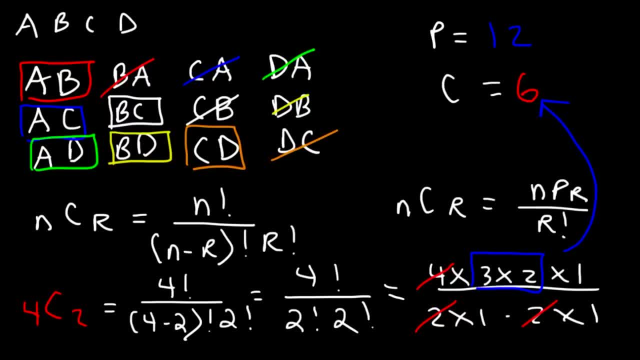 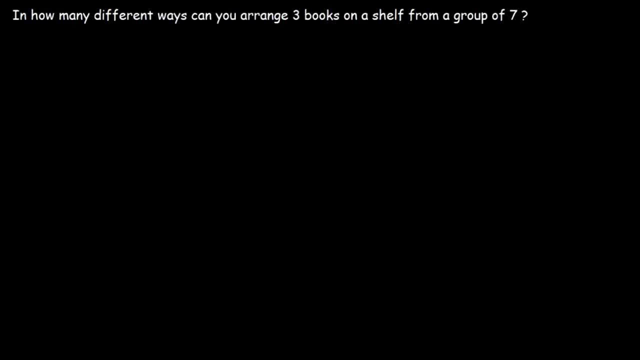 use the equation and also you understand how to make a list to determine the number of permutations and combinations. so now let's work on some example problems. in how many different ways can you arrange three books on a shelf from a group of seven? now go ahead and try. 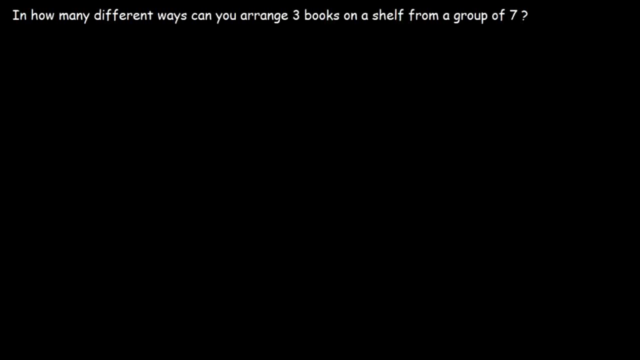 this problem. pause the video, take a minute and feel free to work on it, and then unpause it to see the solution. so is it a permutation or combination? does the order matter? Whenever you see the keyword arrange, typically it's a permutation. The order is important. 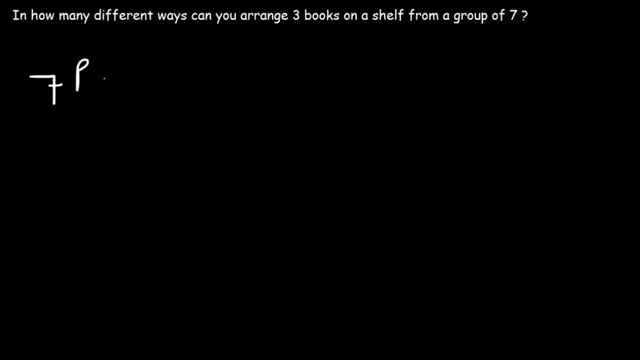 So what we need to write is 7P3.. We're choosing three books from a group or from a total of seven. So this is going to be 7 factorial divided by the difference between 7 and 3.. 7 factorial is 7 times 6 times 5 times 4 times, 3 times, 2 times 1.. 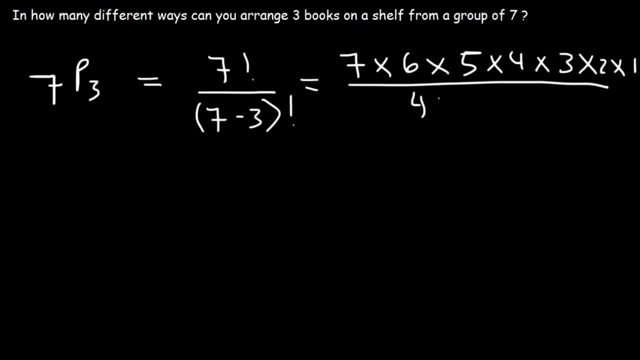 7 minus 3 is 4, and 4 factorial is 4 times 3 times 2 times 1.. So we can cancel these numbers, leaving behind 7 times 6 times 5.. Now, 6 times 5 is 30.. 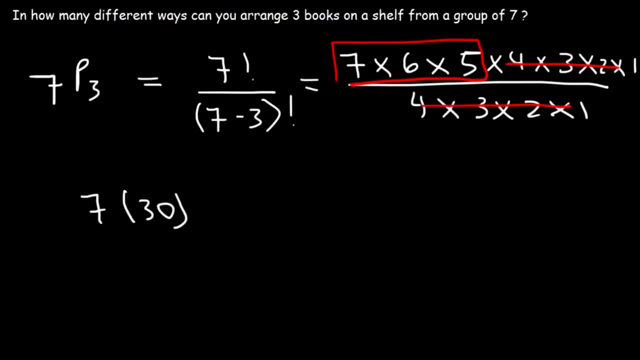 And we know that 7 is 30. And we know that 7 is 30. And we know that 3 times 7 is 21.. So 30 times 7 is 210.. This is the answer. In how many different ways can we arrange five books on a shelf? 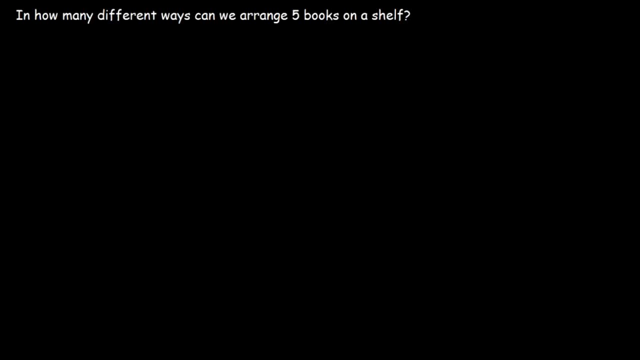 How is this problem different from the last problem And is it still a permutation? Well, we're still trying to arrange books, so the order matters. It's still a permutation, But you can use the fundamental counting principle to get the answer. So we want to arrange five books on a shelf. 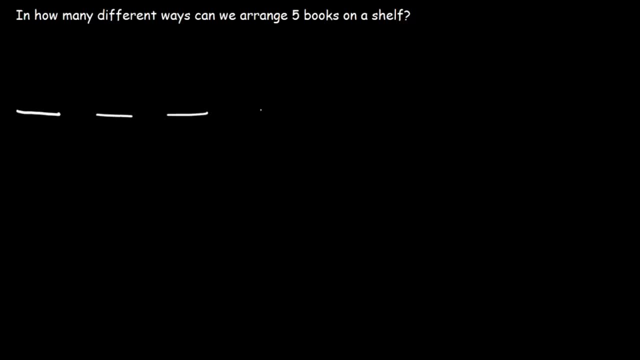 So we want to arrange five books on a shelf Right. So there's five positions. to place the five books In the first position, we can choose any of those five books. So we have five options. Now, once we place the first book in the first position, there's four books left over to choose from. 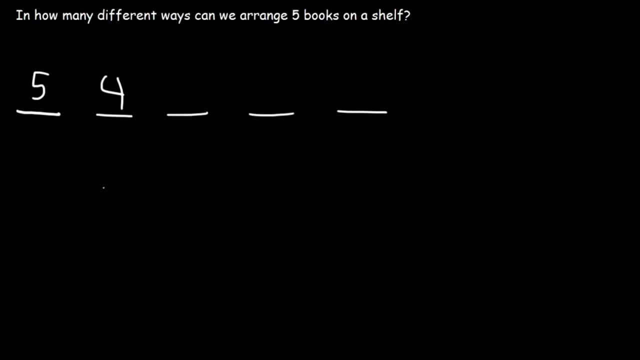 So we can put any of the four books in the second position. Now that we've placed two books, we have three left over, So we can put any of those three books in the third position. Now we have two books left over. 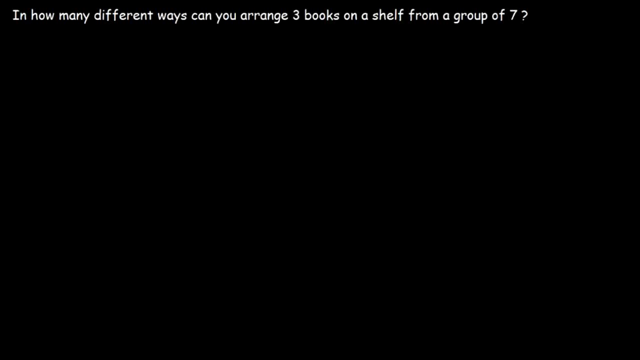 and try this problem. Pause the video, take a minute and feel free to work on it, And then unpause it to see the solution. So is it a permutation or a combination? Does the order matter? Whenever you see the keyword arrange, typically it's a: 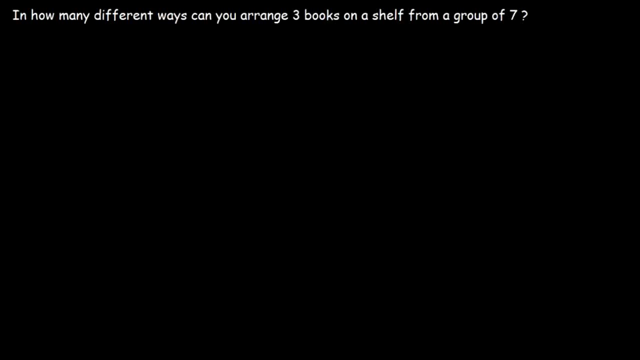 permutation. The order is important, So what we need to write is 7p3.. We're choosing three books from a group or from a total of seven. So this is going to be 7 factorial divided by the difference between 7 and 3.. 7 factorial is 7 times. 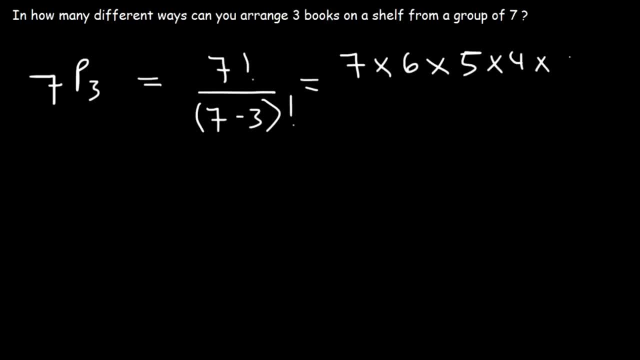 6 times 5 times 4 times 3 times 2 times 1.. 7 minus 3 is 4, and 4, factorial, is 4 times 3 times 2 times 1.. So we can cancel these numbers, leaving behind 7 times 6 times 5.. Now, 6 times 5 is 30, and we 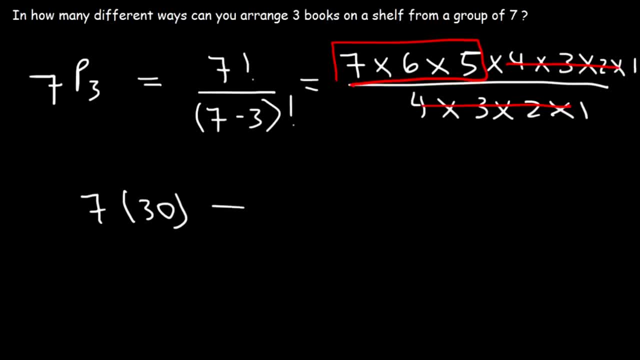 know that 3 times 7 is 21,, so 30 times 7 is 210.. This is the answer. In how many different ways can we arrange five books on a shelf? And you can find that in the on the shelf. How is this problem different from the last problem And is it still a? 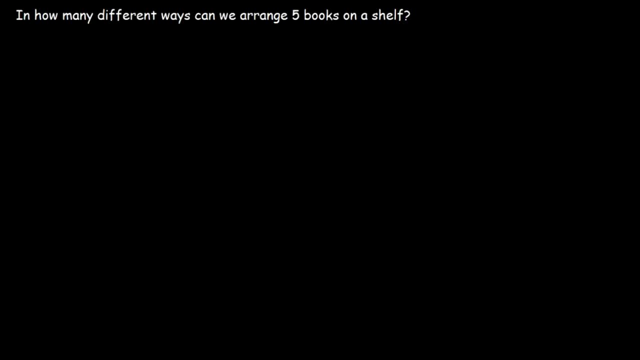 permutation. Well, we're still trying to arrange books, so the order matters. It's still a permutation, But you can use the fundamental counting principle to get the answer. So we want to arrange five books on the shelf, right? So there's five. 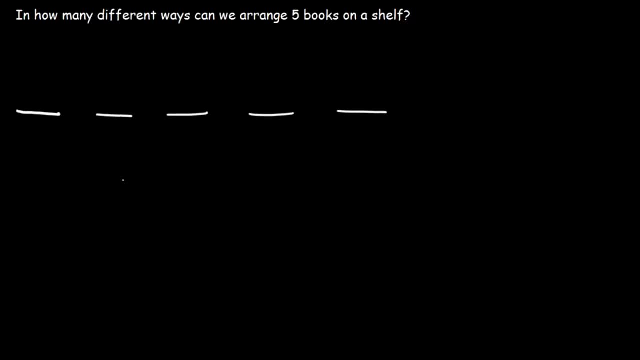 positions. to place the five books In the first position, we can choose any of those five books, So we have five options. Now, once we place the first book in the first position, there's four books left over to choose from, So we can put. 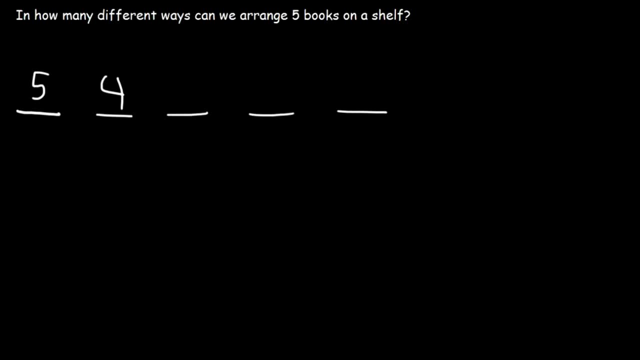 any of the four books in the second position. Now that we've placed two books, we have three left over, So we could put any of those three books in the third position. Now we have two books left over, So we could put any of those two in the 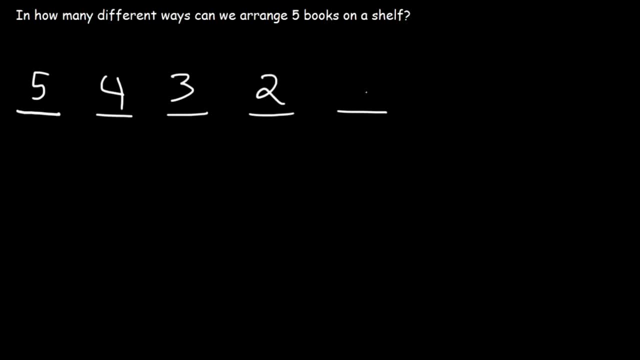 So we can put any of those two in the second to last position, And in the last position we can only put the last book there. So it's going to be five times four times three times, two times one, And that's another way in which you can solve these problems. 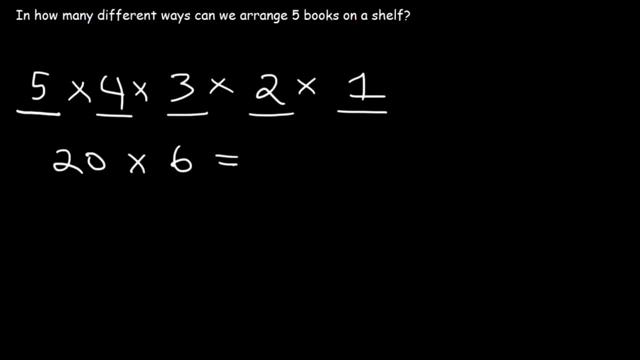 Five times four is twenty. Three times two is six. If two times six is twelve, twenty times six is one twenty. Now, in terms of a permutation, here's how you can calculate it. First, you need to find out what is the total number of books. 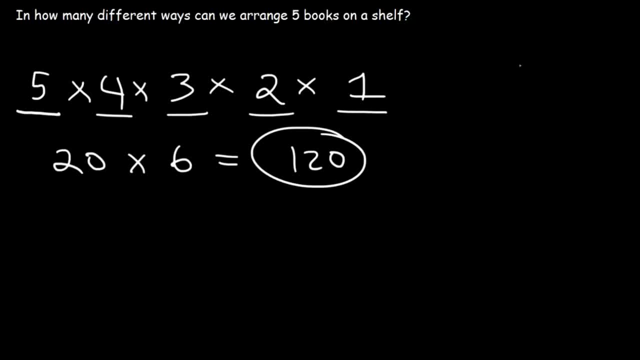 In this problem we only have one number. The total number of books is five And we're choosing all five books from a group of five, So it's going to be five p five, Using the formula npr, is equal to n factorial over n minus r factorial. 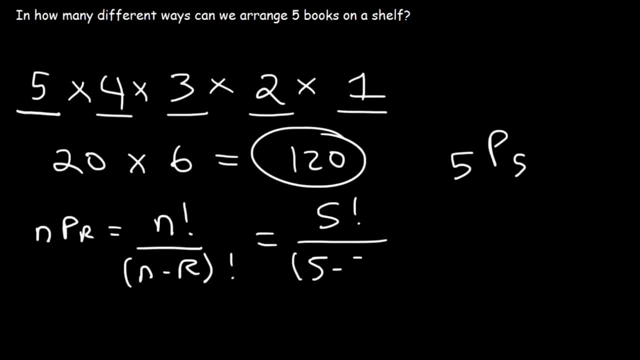 n is five, But r is five as well, So this is going to be five factorial over zero factorial. Now, this is not undefined. Zero factorial does not equal zero. Zero factorial equals one. Make sure you know that. That's just something to know. 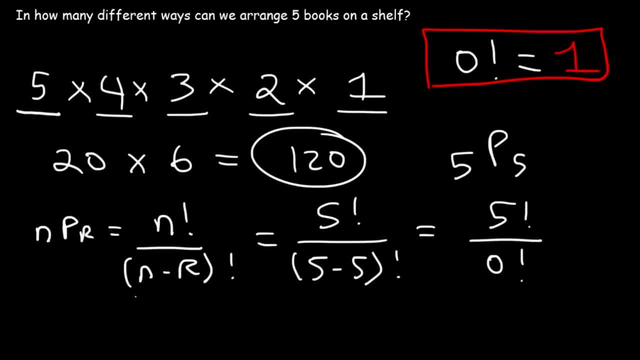 If you're wondering why that's just the way it is. I don't have an answer for you. So this is going to be five factorial over one, And we know that five factorial is five times four times three times two, And this is equal to one twenty. 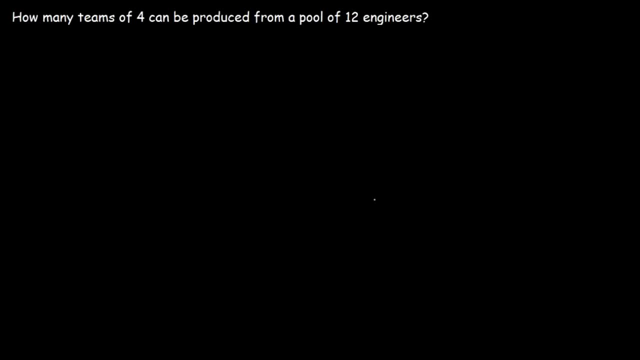 How many teams of four can be produced from a pool of twelve engineers? So is this a permutation or is it a combination? What do you think? Does the order matter? So let's say, if I select four individuals- John, Sue, Sally and Chris- 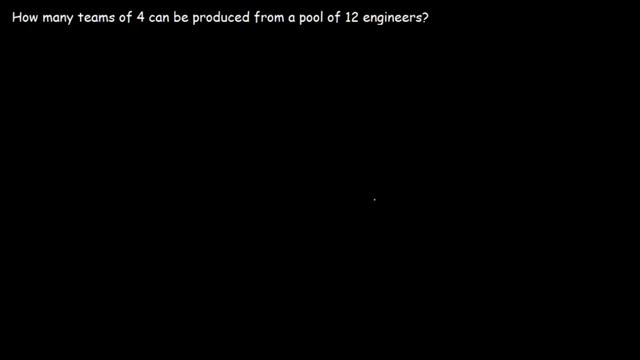 Does it really matter if I select John, Chris, Sally, Sue, It's the same team of four, So in this problem, the order doesn't matter. Therefore, it's a combination. So we're choosing four from a total of twelve. 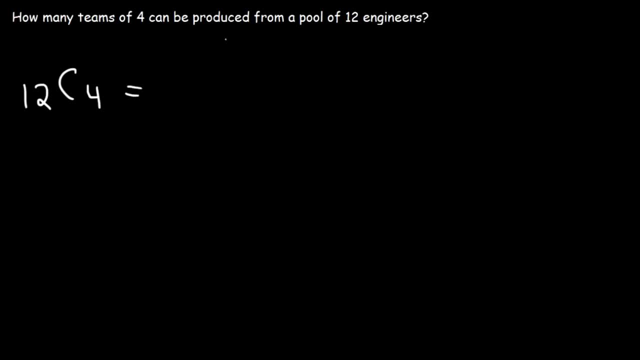 So it's going to be twelve c four, And this is equal to n factorial or twelve factorial divided by n minus r factorial, That's twelve minus four factorial times, r factorial or four factorial. So twelve minus four Is equal to eight. 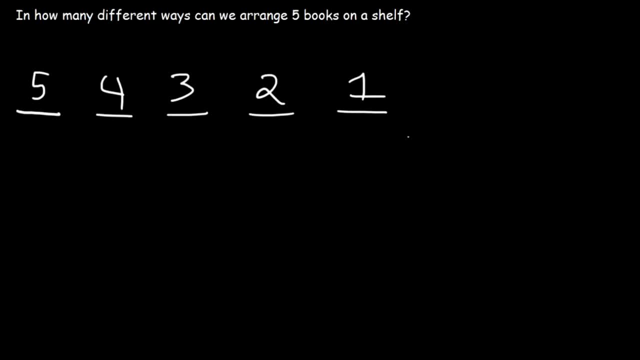 second to last position, And in the last position we can only put the last book there. So it's going to be five times four times three times two times one, And that's another way in which you could solve these problems. Five times four is 20.. Three. 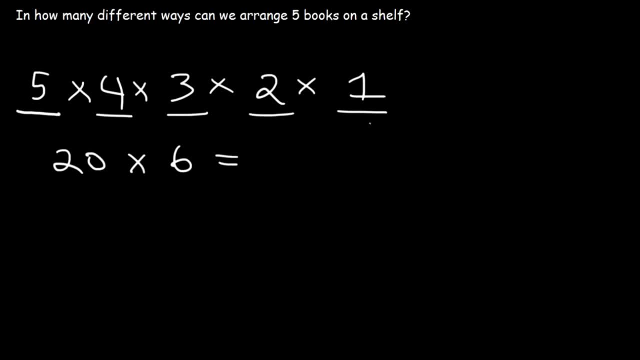 times two is six. If two times six is 12,, 20 times six is 120.. Now, in terms of a permutation, here's how you can calculate it. First, you need to find out what is the total number of books. In this problem, we only have one number: The total. 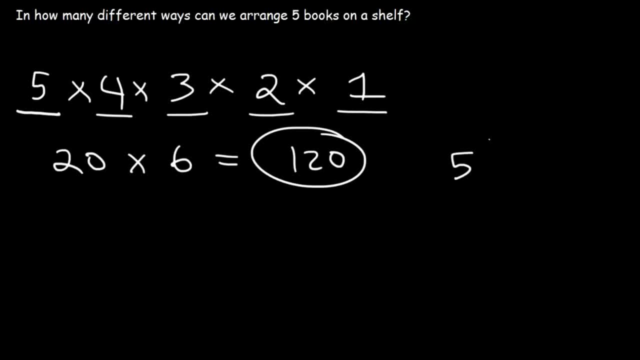 number of books is five And we're choosing all five books from a group of five, So it's going to be 5p5.. Using the formula, npr is equal to n factorial over n minus r. factorial n is five, but r is five as well, So this is going to be five factorial over zero. 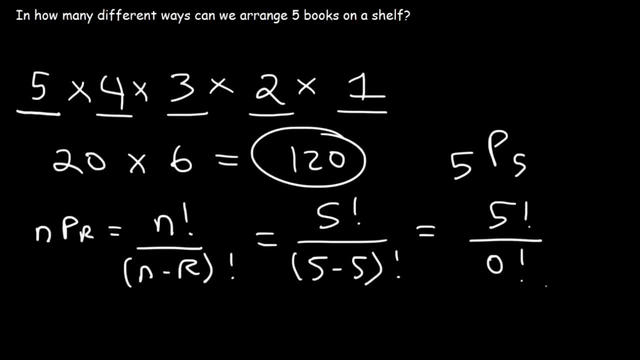 factorial. Now, this is not undefined. Zero factorial does not equal zero. Zero factorial does not equal zero. zero factorial does not equal zero. Zero factorial equals one. Make sure you know that. That's just something to know. If you're wondering why, that's just the way it is. I don't have an answer for you. 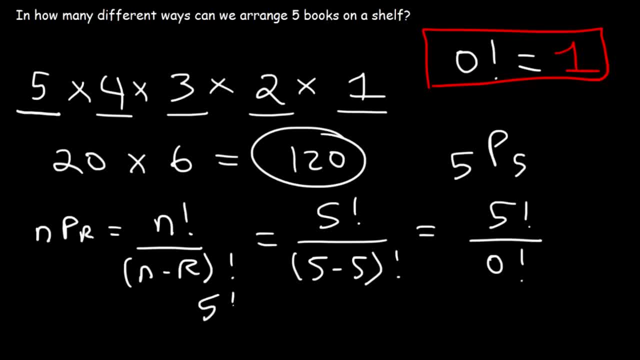 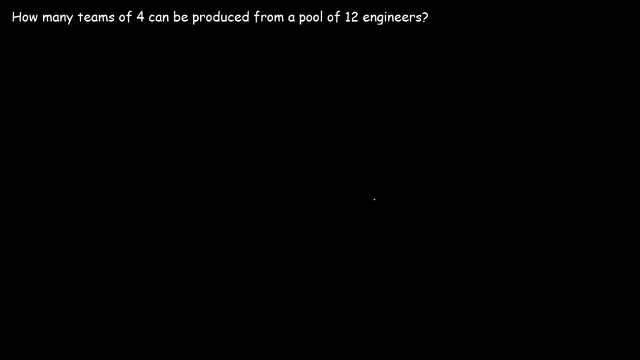 So this is going to be five factorial over one, And we know that five factorial is five times four times three times two times one, And this is equal to 120.. How many teams of four can be produced from a pool of 12 engineers? So is this a? 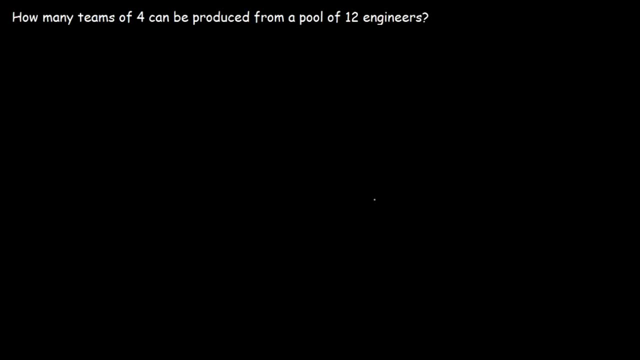 permutation or is it a combination? What do you think? Does the order matter? So let's say, if I select four individuals- John, Sue, Sally and Chris- Does it really matter? if I select John, Chris, Sally, Sue, It's the same team of four. So in this, 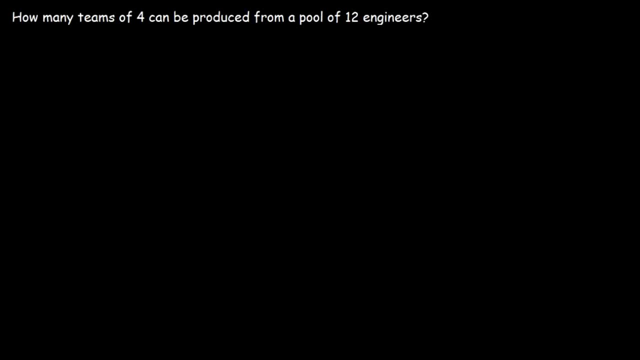 problem. the order doesn't matter. Therefore it's a combination. So we're choosing four from a total of 12.. So it's going to be 12c4.. And this is equal to n factorial, or 12 factorial divided by n minus r factorial, That's 12 minus 4 factorial times r factorial, or. 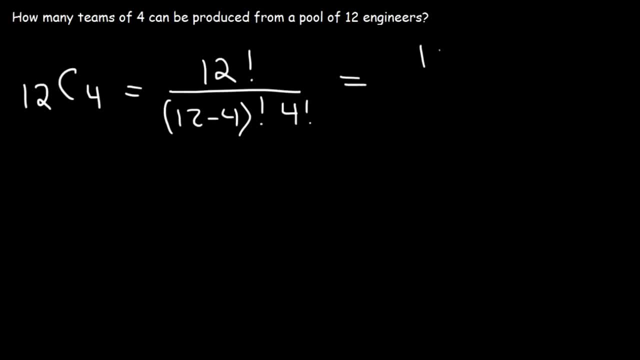 four factorial. So 12 minus 4 is equal to 8.. Now, if you don't want to write 12 times 11 times 10 times, 9 times, 8 times 7, all the way to one, Here's what you can do. Notice that you have an 8 factorial on the bottom. 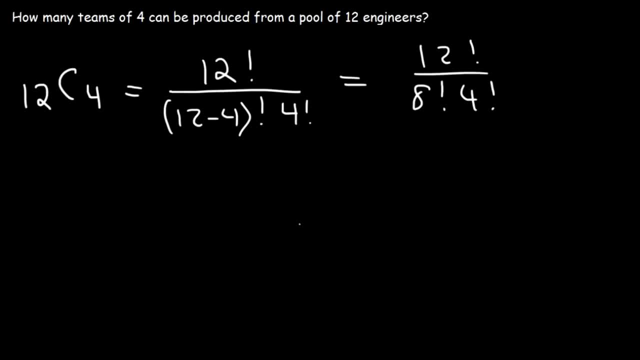 So you want to write 12 just before you get to 8.. So 12 factorial is 12 times 11 times 10 times 9 times 8 factorial, Because 8 factorial will go from 8 to 1. And you don't need to write all of it. Stop at 8 factorial because we can. 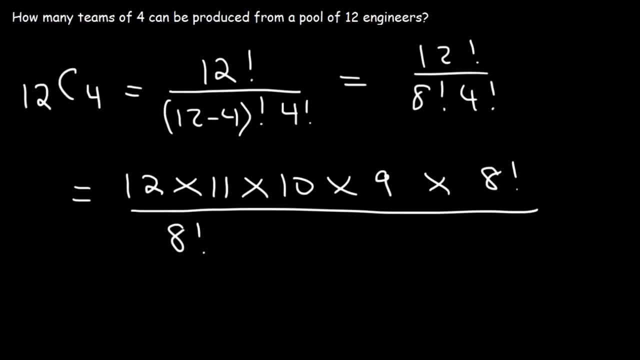 cancel it in the next step. Now 4 factorial- I'm going to write that out: That's 4 times 3 times 2 times 1.. So let's cancel 8 factorial. That's going to save us some writing space. 4 times 3 is 12.. So we can get rid. 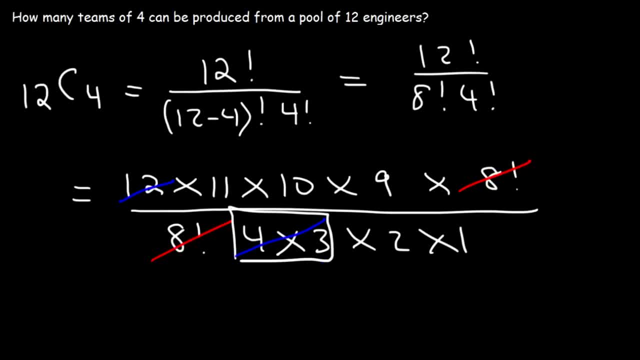 of these two, And then 10 divided by 2 equates to 5.. So what we now have is 11 times 5 times 9.. 11 times 9 is 99.. Now what is 99 times 5?? 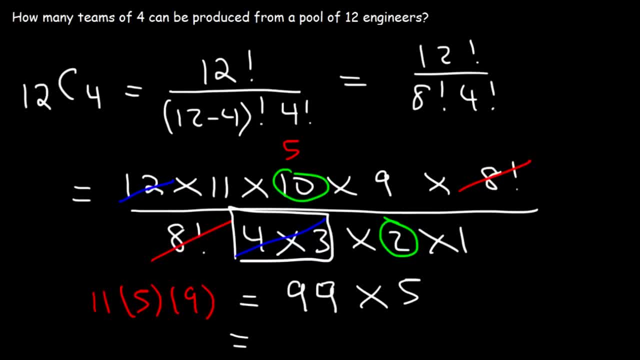 Well, if you want to do that without your calculator, think of it this way: 99 is 100 minus 1.. Let's distribute: 100 times 5 is 500.. 5 times 1 is 5.. 500 minus. 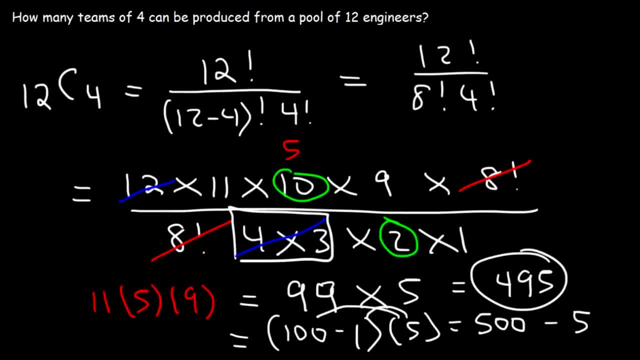 5 is 495.. And so we can choose 495 teams of 4 from a pool of 12 engineers, And so that's it for this video. Thanks for watching. If you want to find more videos that I've created in algebra, trig, pre-cal calculus, chemistry and physics, just visit my channel and 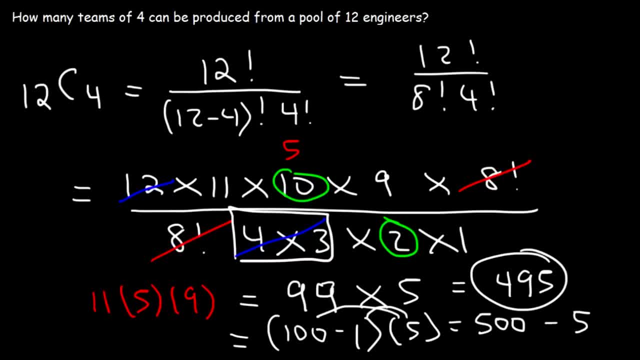 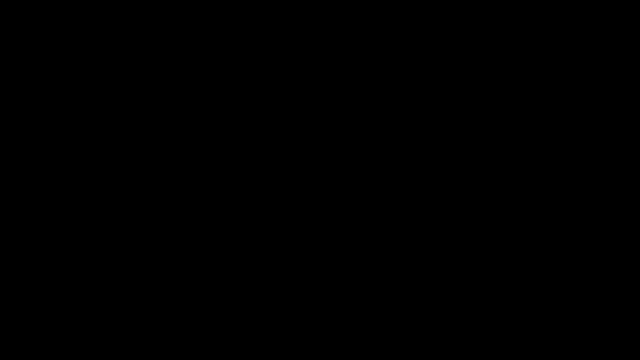 you can find my playlist on those topics. Well, I changed my mind. I just realized that there are some other problems that I need to go over that's related to this topic. How many different ways can you arrange the letters in the word Alabama? This is: 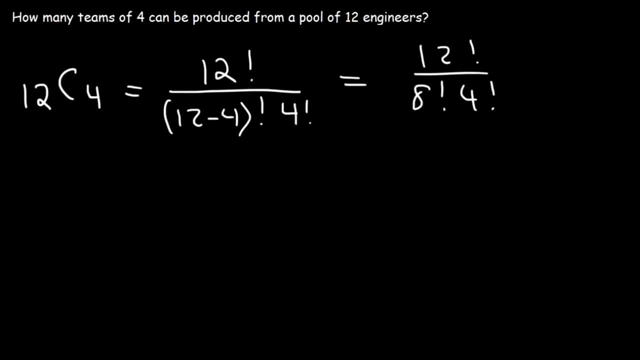 Now, if you don't want to write twelve times, eleven times ten times, nine times, eight times seven, all the way to one, here's what you can do. Notice that you have an eight factorial on the bottom, So you want to write twelve just before you get to eight. 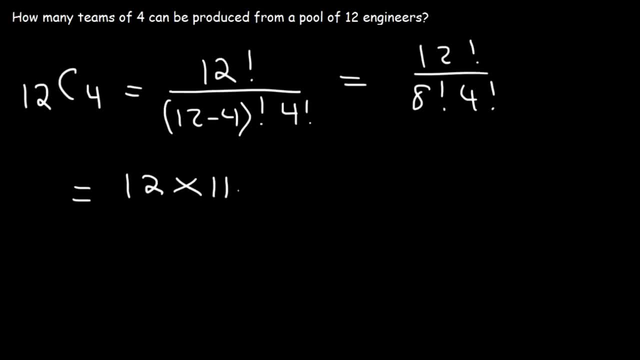 So twelve factorial is twelve times eleven times ten times nine times eight factorial, Because eight factorial will go from eight to one And you don't need to write all of it. Stop at eight factorial, because we can cancel it in the next step. 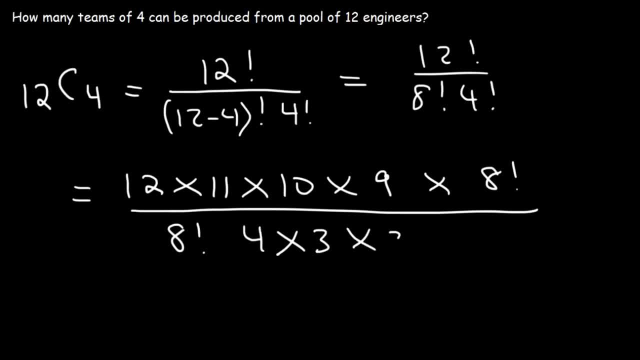 Now four factorial- I'm going to write that out. That's four times three times two times one. So let's cancel eight factorial. That's going to save us some writing space. Four times three is twelve, So we can get rid of these two. 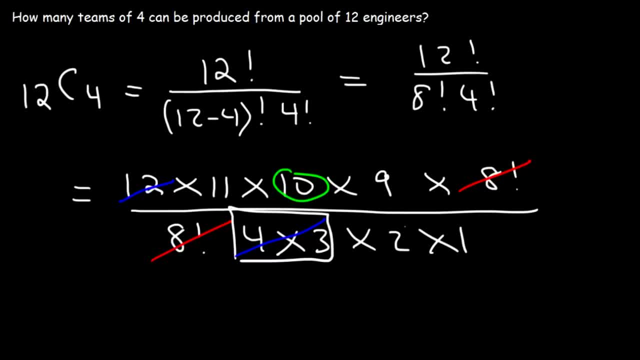 And then ten divided by two equates to five. So what we now have is eleven Eleven times nine is ninety-nine. Now, what is ninety-nine times five? Well, if you want to do that without your calculator, think of it this way: 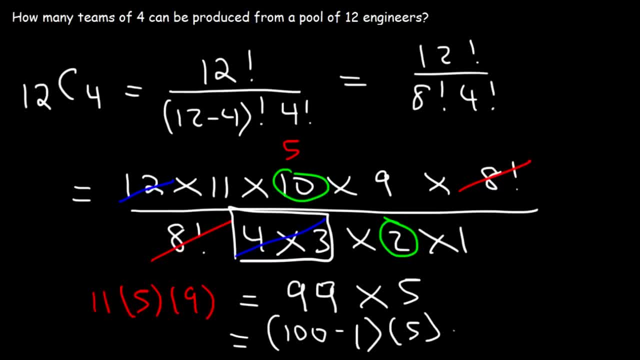 Ninety-nine is a hundred minus one. Let's distribute: A hundred times five is five hundred. Five times one is five. Five hundred minus five is four, ninety-five, 495.. And so we can choose 495 teams of four from a pool of 12 engineers, And so that's it for this. 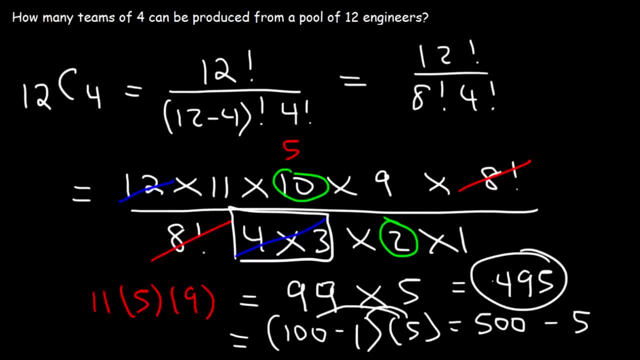 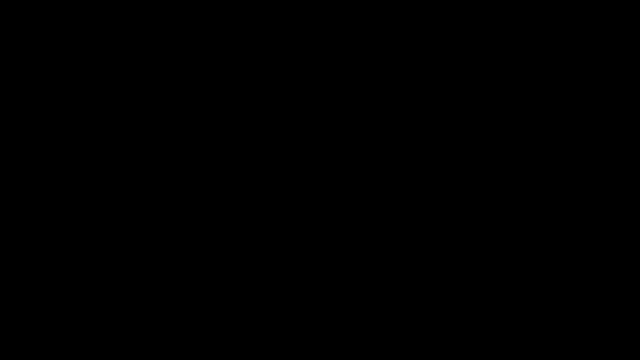 video. Thanks for watching. If you want to find more videos that I've created in algebra, trig, pre-cal calculus, chemistry and physics, just visit my channel and you can find my playlists on those topics. Well, I changed my mind. I just realized that there are some other problems that 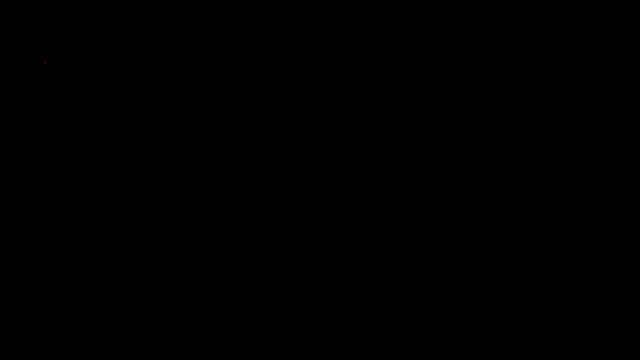 I need to go over that's related to this topic. How many different ways can you arrange the letters in the word Alabama? This is a very common question that you might see in this type of topic, And here's what you need to do. First, count the number of letters that are in the word Alabama. 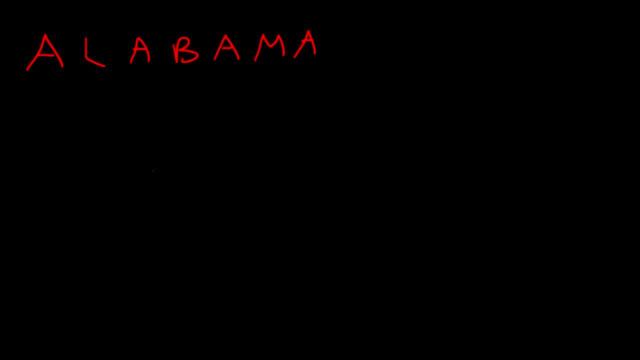 a very common question that you might see in this type of topic, And here's what you need to do. First, count the number of letters that are in the word Alabama. There's a total of seven letters, So it's going to be 7 factorial on the top of. 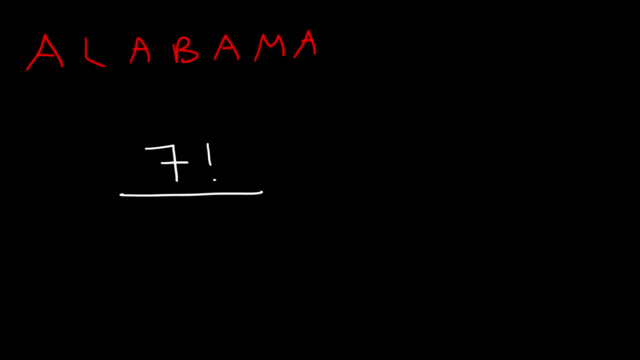 the fraction and on the bottom divide, by the letters that repeat. There's only one letter that repeats and it's A, And A repeats four times. So we're going to divide it by 4 factorial. So therefore this is going to be 7 times, 6 times, 5 times 4 factorial divided by 4 factorial. And so we could. 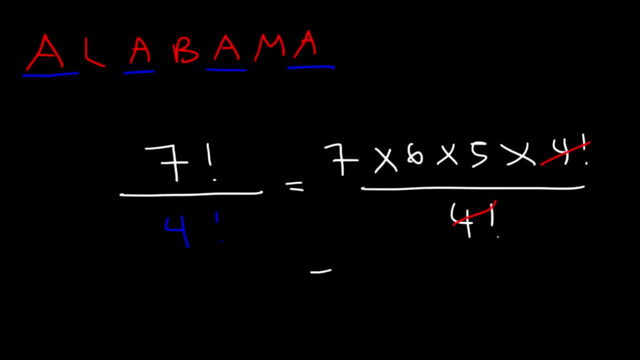 cancel these two. We know that 6 times 5 is 30 and 7 times 30 is 210.. So that's how many different ways you can arrange the letters in the word Alabama. Let's try another example. What about the word Mississippi? In class I've seen this a lot, so it's a very 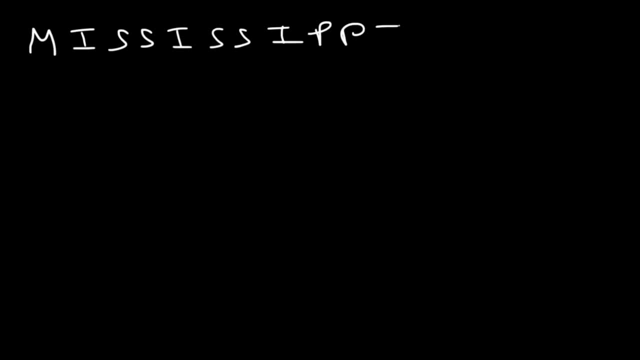 common example, So I'm going to use it. So first let's count how many letters that we have. There's a total of 11 letters, So it's going to be 11 factorial on top divided by Now. let's find the letters that repeat. I repeats four times. So we're. 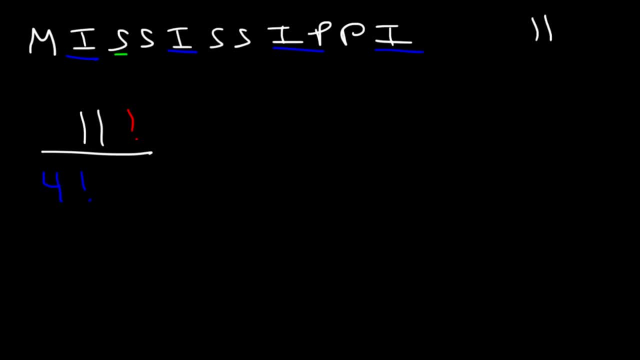 going to divide it by 4 factorial. S repeats four times, So another 4 factorial, And P repeats twice, So 2 factorial. So this is going to be 11 times, 10 times, 9 times, 8 times, 7 times, 6 times, 5 times 4 factorial divided. 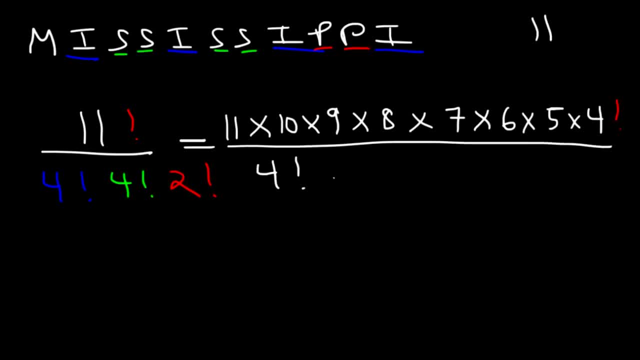 by. I'm going to leave the first 4 factorial the same- I'm not going to change it- And the other 4 I'm going to write as as 4 times 3 times 2 times 1, and then 2 factorial 2 times 1.. So we can cancel 4 factorial And let's see what else. 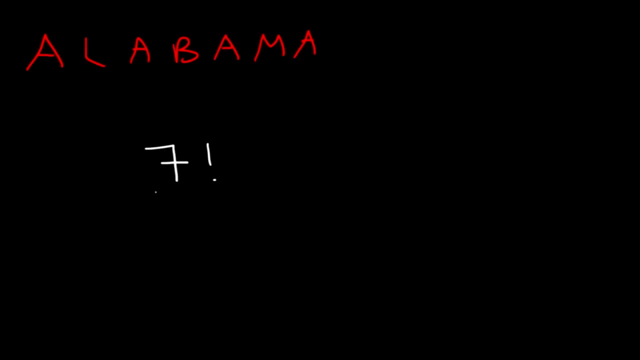 There's a total of seven letters, So it's going to be seven factorial. on the top of the fraction and on the bottom divide by the letters. There's only one letter that repeats, and it's a, and a repeats four times. So we're going to divide. 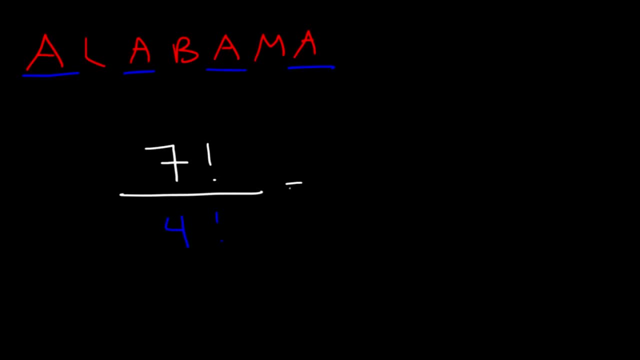 it by four factorial. So therefore this is going to be seven times six times five times four factorial, divided by four factorial, And so we could cancel these two. We know that six times five is 30 and seven times 30 is 210.. So that's how many different ways you can arrange the letters. 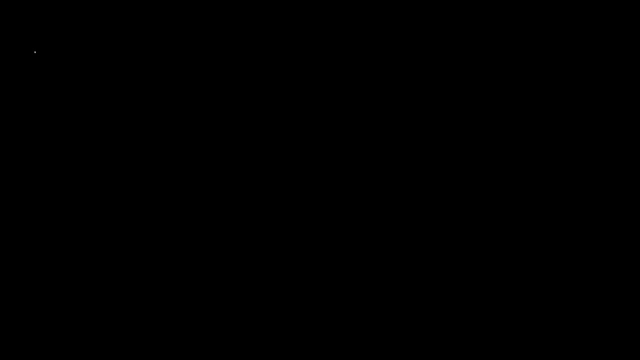 In the word Alabama. Let's try another example. What about the word Mississippi? In class I've seen this a lot, So it's a very common example, So I'm going to use it. So first let's count how many letters that we have. 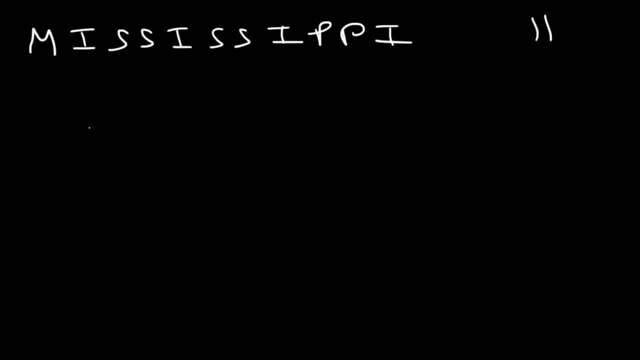 There's a total of 11 letters, so it's going to be 11 factorial on top Divided by. Now let's find out how many letters we have. Find the letters that repeat- I repeats four times. so we're going to divide it by four: factorial. 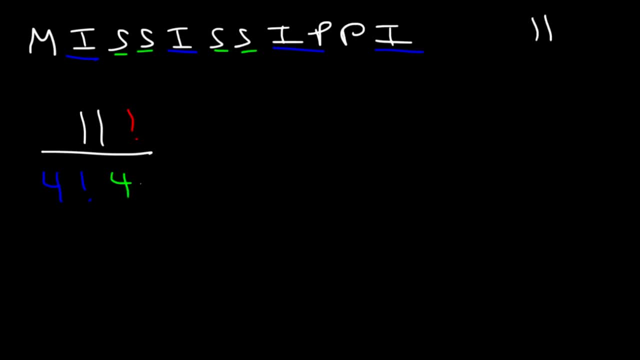 S repeats four time, So another four factorial, And P repeats twice, So two factorial. So this is going to be 11 times 10 times nine times, eight times, seven times, six Times, five times four factorial Divided by. I'm going to leave the first four factorial the same. I'm not going to change it. 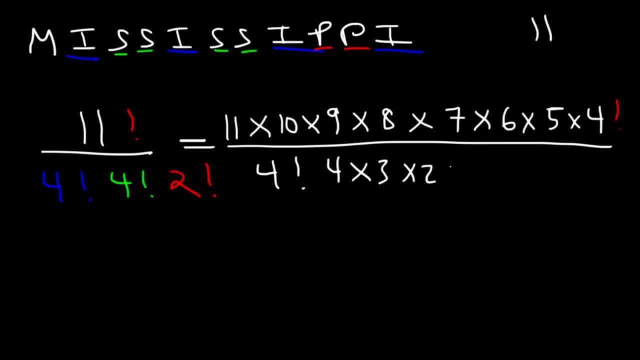 And the other four. I'm going to write it as four times three times two times one, And then two factorial, two times one. So we can cancel four factorial. And let's see what else can we cancel. Well, we know that Three times two is equal to six.